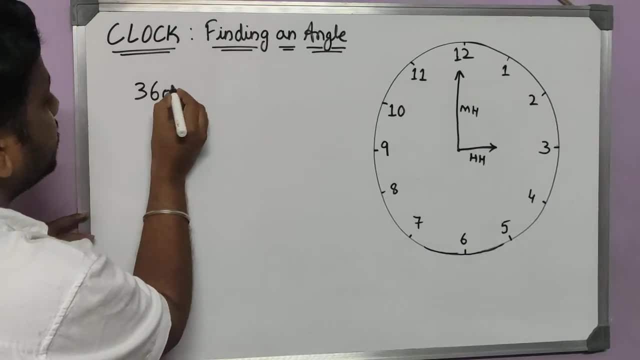 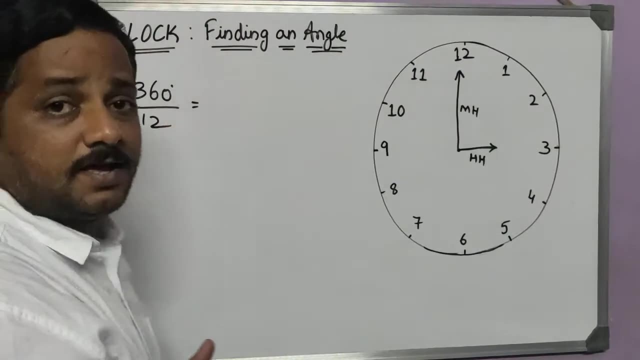 hand has to rotate for 360 degree. So in that 360 degree, each sector means we have 12 sectors. So when I divide that 360 by 12, we will get an angle of each sector. Okay, so the angle of each. 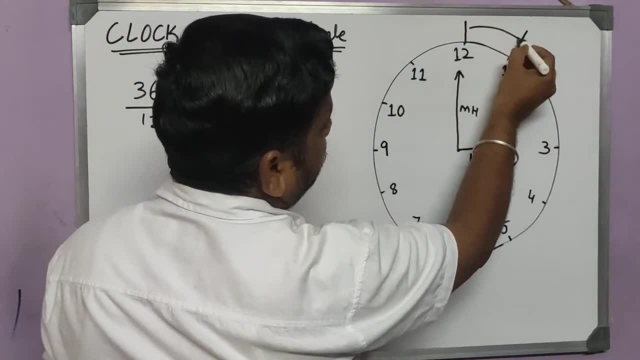 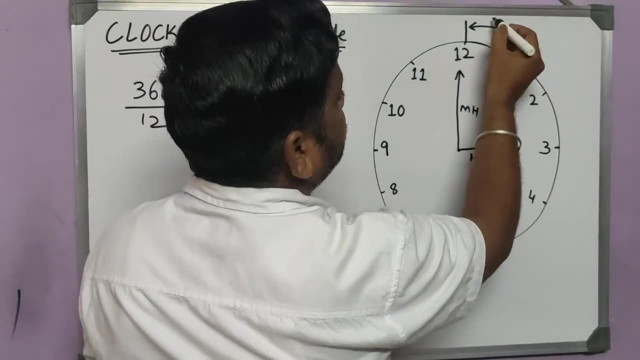 sector means what is an angle from 12 to 1.. So this we can identify. So 360 by 12 we can say it should be радial to 8, so this angle, here to the maximum extreme, this 0.24 degree, which is 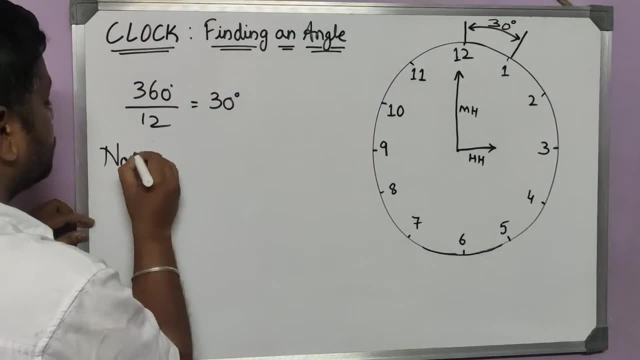 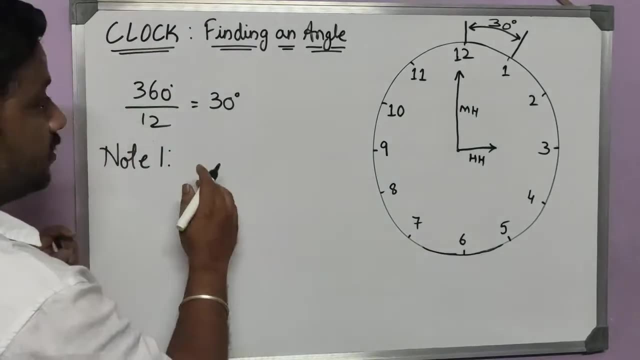 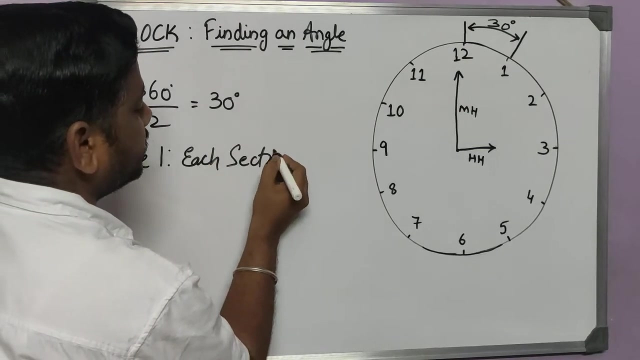 right. once you, it has to be right. so I am going to divide this by 3 or 2.. tuned out the�. everywhere else it 7. so it is right. it does not matter. For depression, let us say seesehen, and, but this can be an angle 0.23. yeah, and then the second aspect that we are going to consider: each sector spicy gehent. So this is the mains hand we want to put, as 30 degree means each sector is govin to have an angle of 30degrees. This is an important point, so note this and we 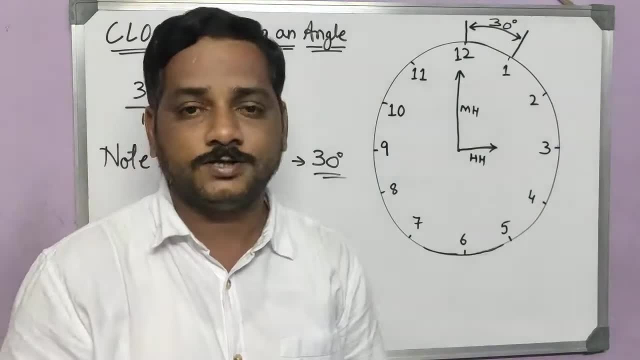 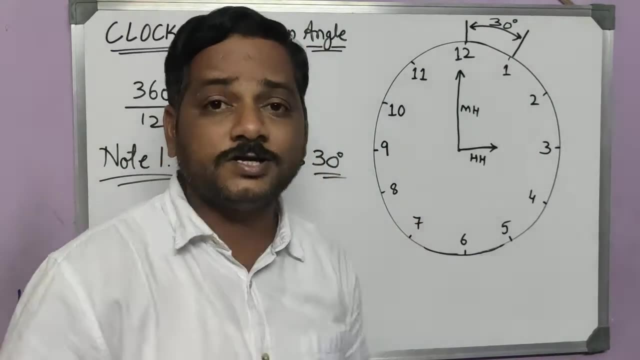 1 to 1, it is 30.. 1 to 2, it is 30.. 2 to 3, it is 30.. That is a point. So this is note 1,, most important note, And we have second note that is also important to solve the problem. To understand that second note, let me take an example here. 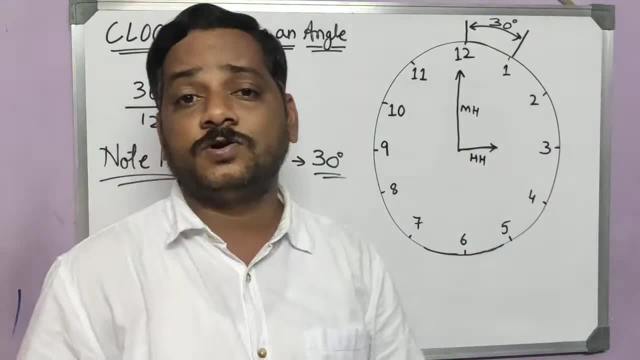 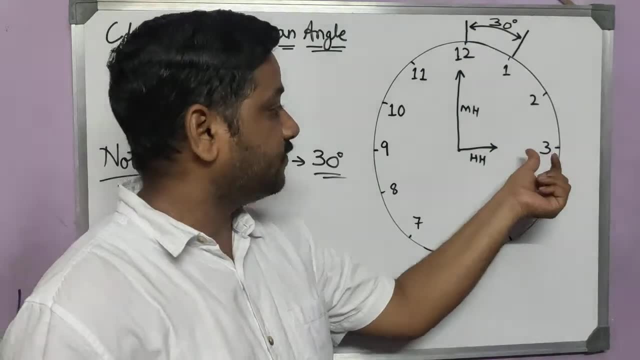 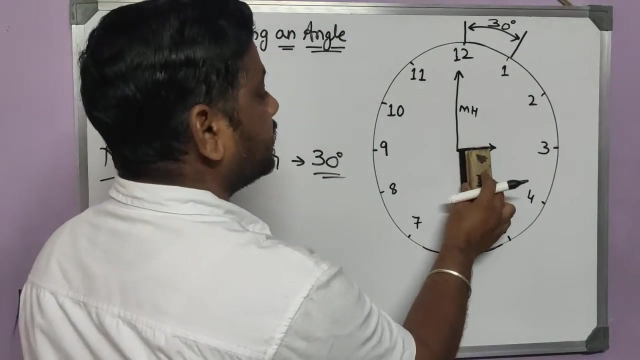 See now, according to this picture it is pointing towards 3 o'clock. Now say this hour there is one hour has been taken Means. I will take that it is changing from 3 to 4. Say the hour hand is moving from 3 to 4. If it is 1 hour, then we can say the time has changed from 3 to 4.. Right, 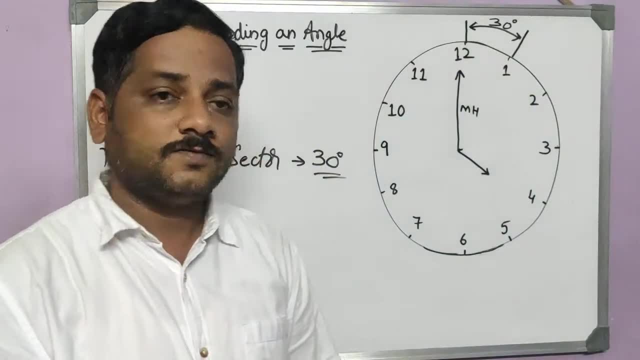 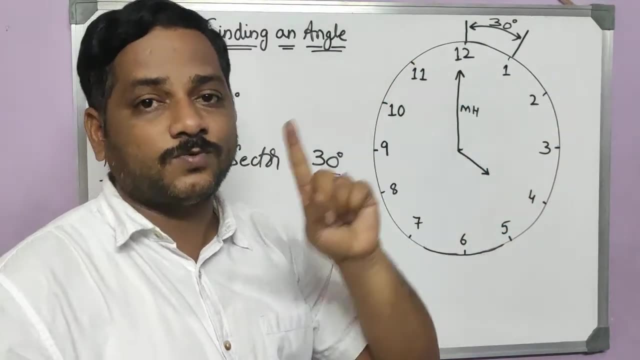 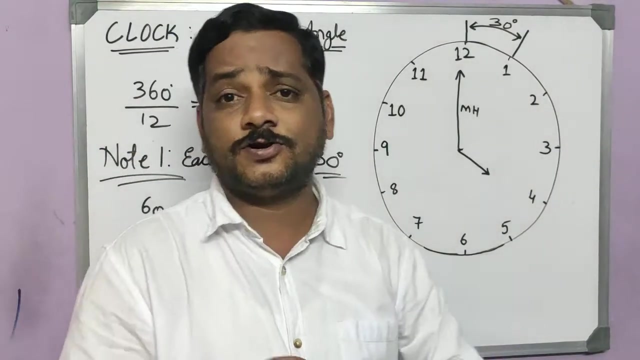 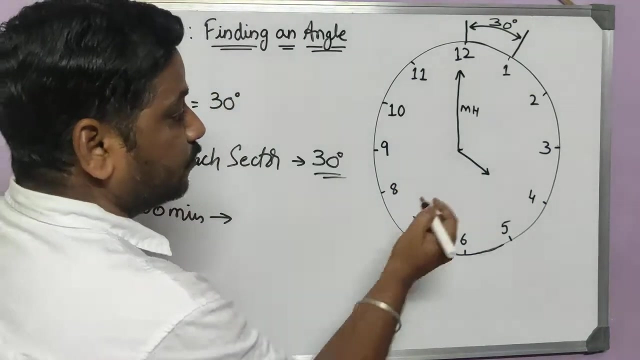 So to have this 1 hour, we know that the minute hand has to give 60. It has to rotate 360 degree to get 1 hour Means for 60 minutes we get 1 hour. That is the basic concept we know. So if minute hand gives a 60 minute, then this hour hand will move from 3 to 4.. 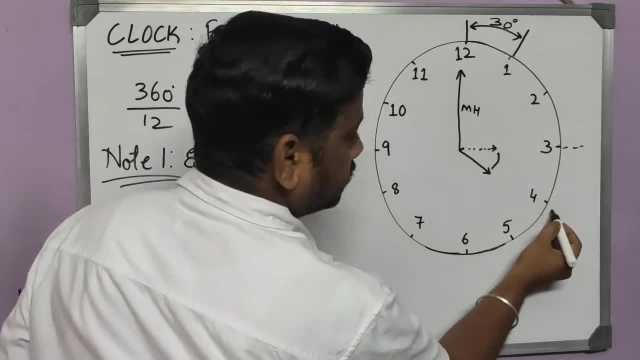 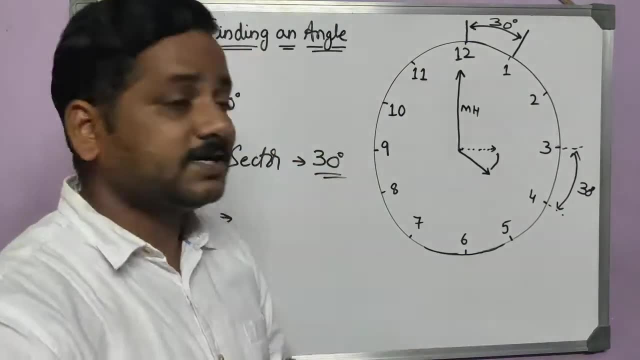 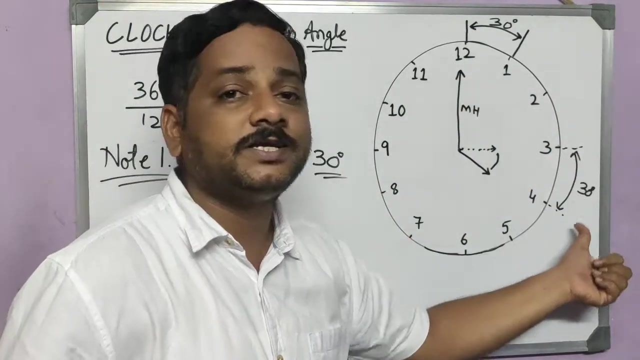 See, hour hand is just moving from this point to this point Means it is just moving 30 degree. So we can say we can relate it like this: If minute hand is moving for 60 minutes, then hour hand will cover only 30 degree. It moves from 1 hour to the next hour. So this angle is 30 degree according to the note 1.. 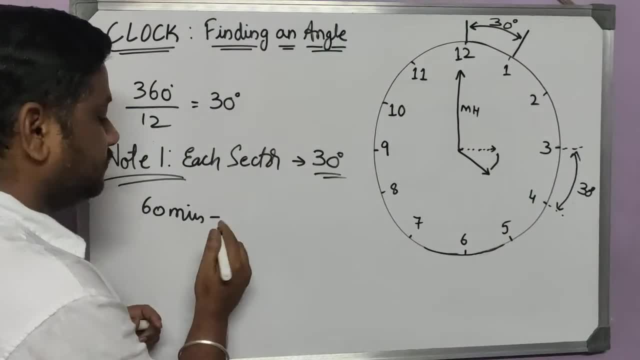 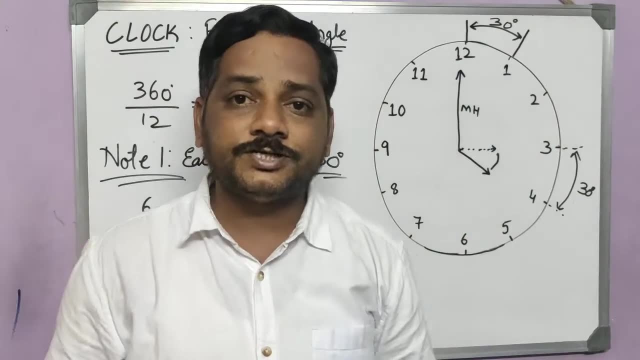 So we can say that if it is a 60 minute, if minute hand is moving for 60 minutes, that is equal to hour hand 30 degree. Okay, So what we are trying to do here is we are trying to relate the movement of both the hands- Minute hands and the hour hand. 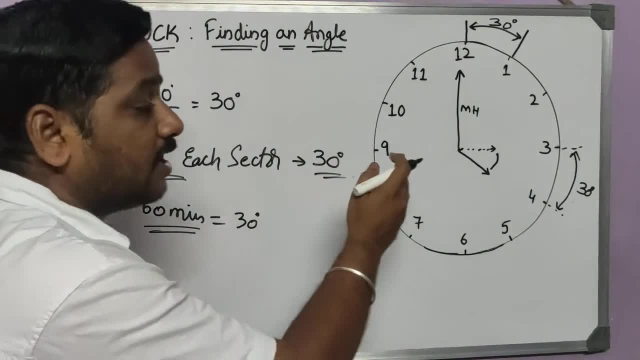 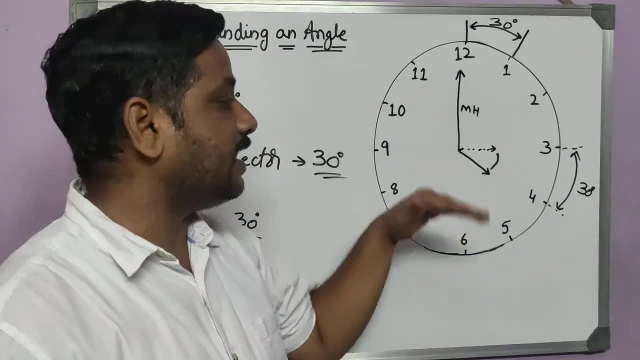 If minute hand moves for 60 minutes, then hour hand will move for just 30 degree. So now, using this, I can identify what would be the angle moved by this hour angle, hour hand if just minute hand is moved for 1 minute. 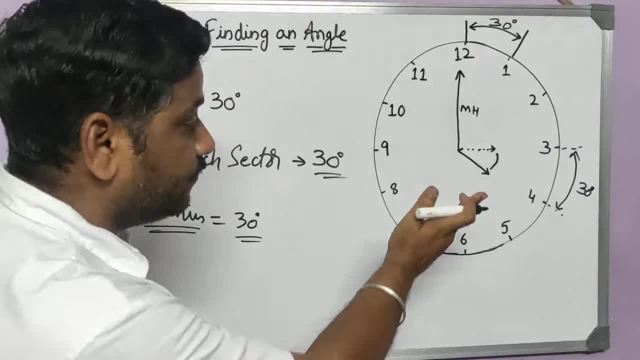 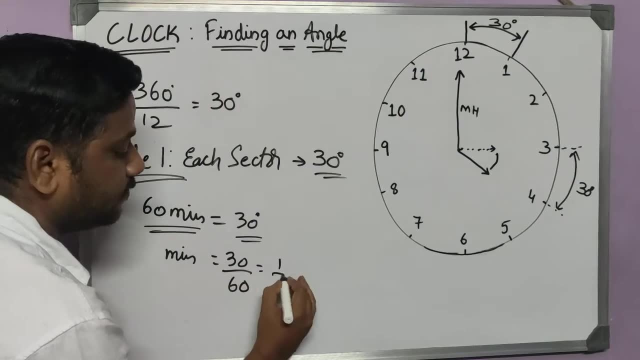 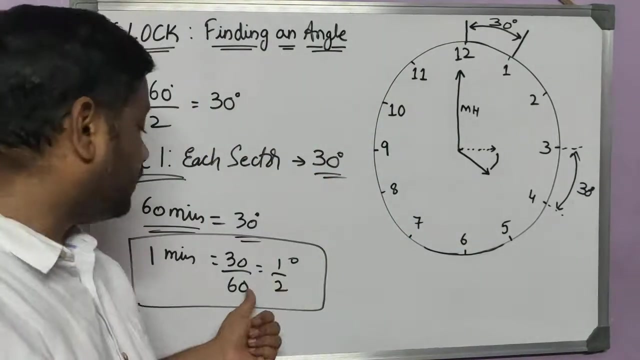 So we can say that if 60 minutes, if it is moving for 30 degree for 1 minute, it is going to be 30 by 60. It is nothing but 1 by 2 degree. So for one minute, if minute hand moves for one minute, then hour hand will move for just half a degree. 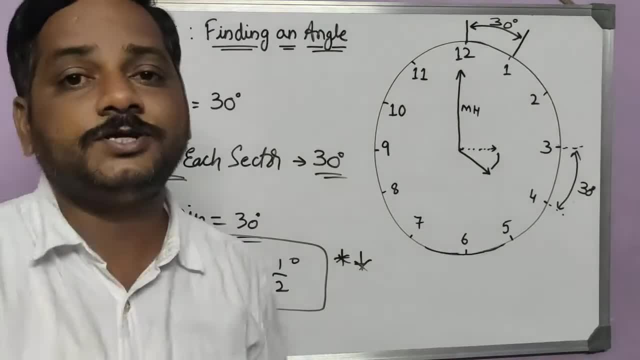 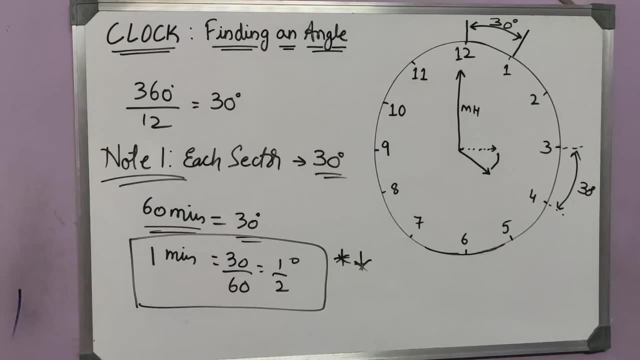 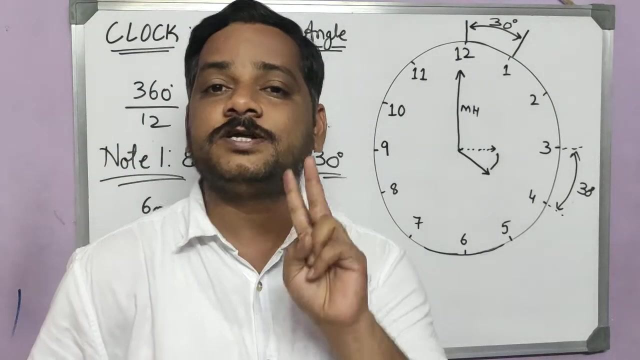 So this is the most important note you need to consider, which will be helpful to solve the problem related to the finding of an angle between the hour hand and minute hand. So I will make it very clear Two important notes we need to consider. 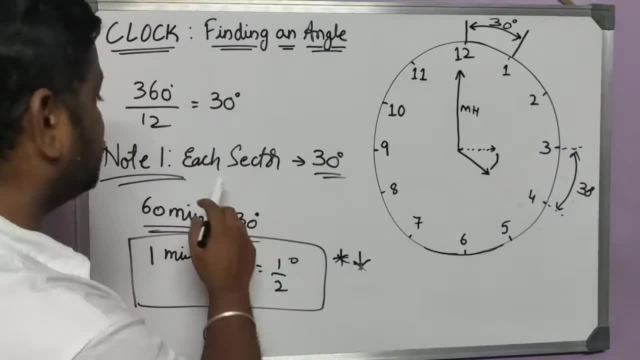 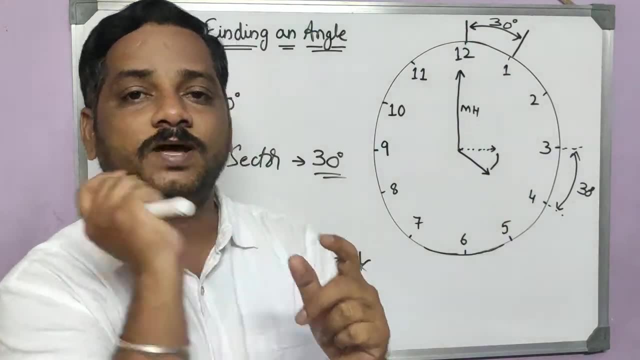 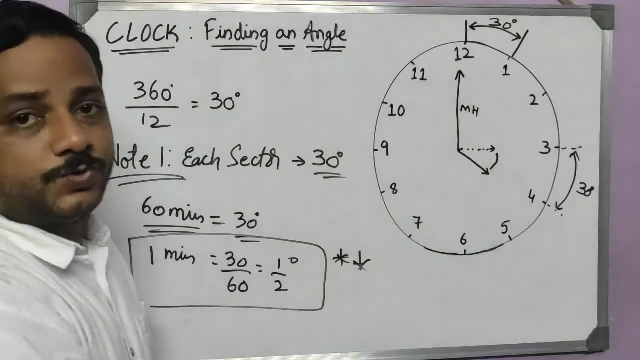 That is, each sector will have a 30 degree and if minute hand moves for one minute hour, hand will just move by half a degree. So for example, say: if minute hand moves for 20 degree, say minute, we have 20 minutes. 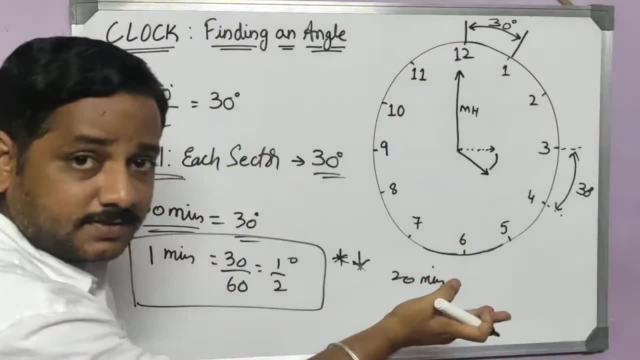 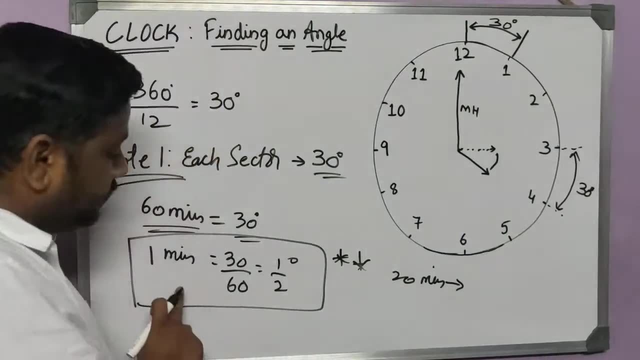 So minute hand is moving from 12 to 4, means 20 minutes. Then how much of hour hand has been moved So that we can just do it like this? For one minute it is half degree, So for 20 minutes it will be 20 by 2, that is 10 degree. 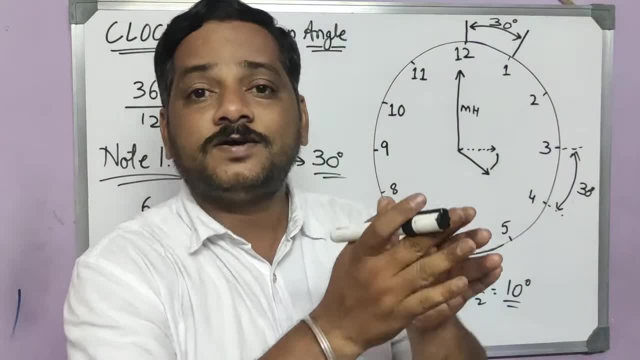 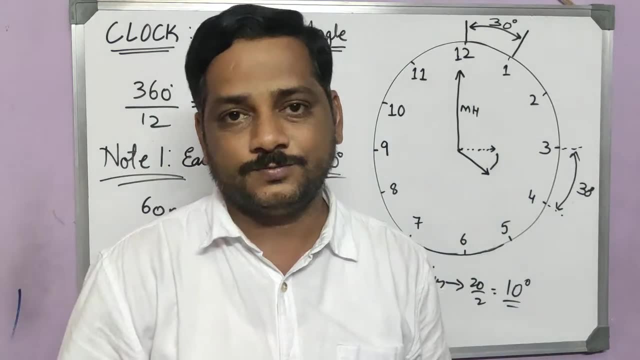 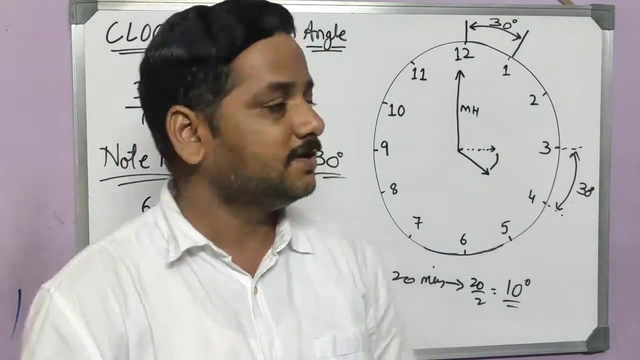 That is how I can find out the moment of hour hand in degrees. So these two notes will help you to solve the problem. Now let us take one or two examples to understand how to find an angle between the minute and hour hand. 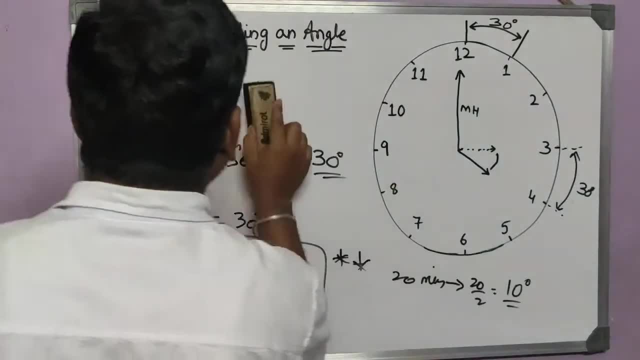 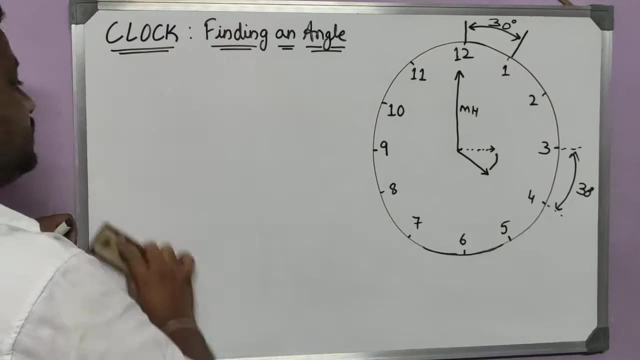 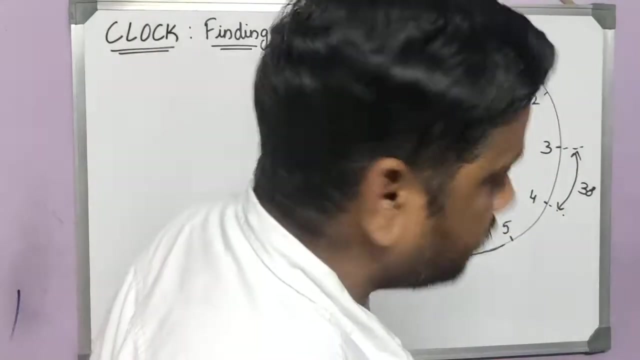 So let me take simple, Let me erase these notes here, But you have to remember these notes so that you can solve it easily. Let us elaborate the examples so that you can understand the concept very easily, comfortably. Say what would be the angle if the time is, say now, 2.40.. 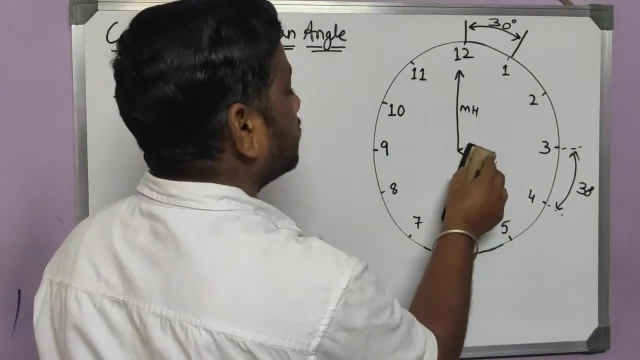 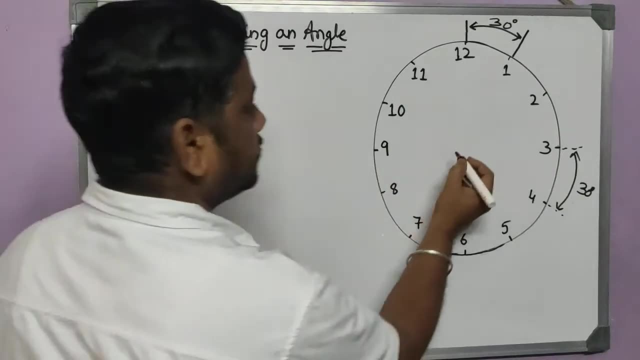 2 o'clock and 40 minutes. So let me change it. Say now the time is 2 over 40 minutes, 2 hours, 40 minutes. So first you just have the picture like this, So that see, for beginners you can draw the picture. 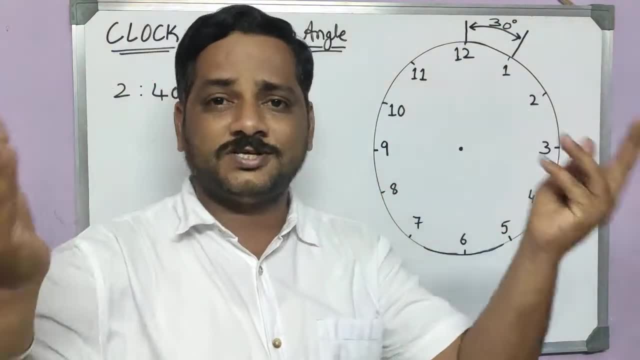 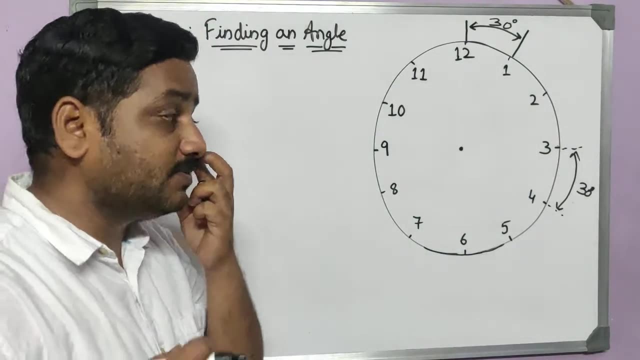 Once you go on practicing the problems later you can have this picture in your mind itself. Okay, Only for the beginners. I am telling you to have this picture So that, while practicing, it will become easy for you to understand. So, 2 o'clock. 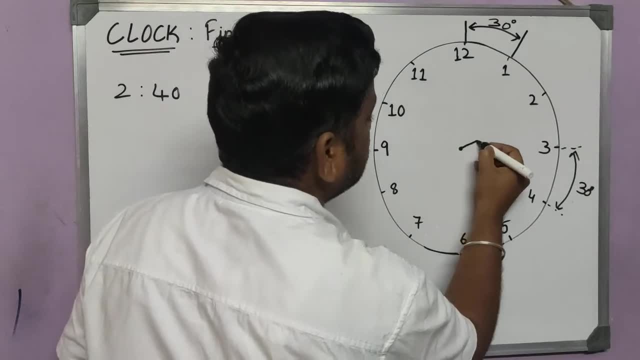 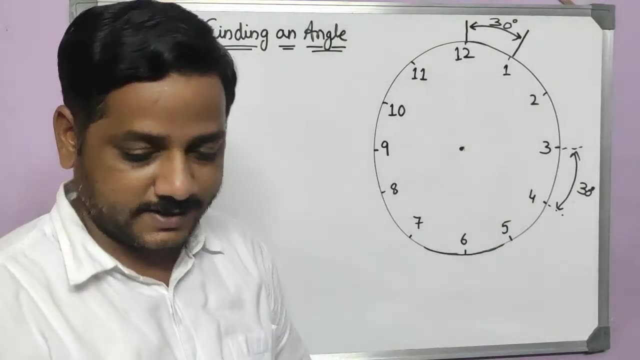 So we can say: the hour hand, Hour hand is nothing but small hand. So the hour hand will be pointing towards Just a minute. Before plotting the hour, First let me show you minute hand. So minute hand is plotting pointing towards 40 minutes. 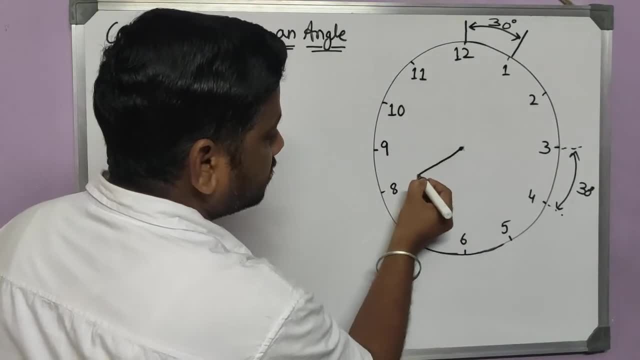 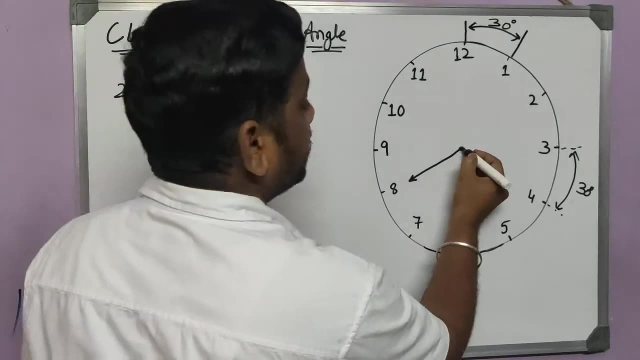 So 40 minutes means it has to point towards 8.. Right, So this is minute hand, But what about the hour hand? Hour hand will not be pointing exactly towards 2.. It will not be pointing towards 2. Why? 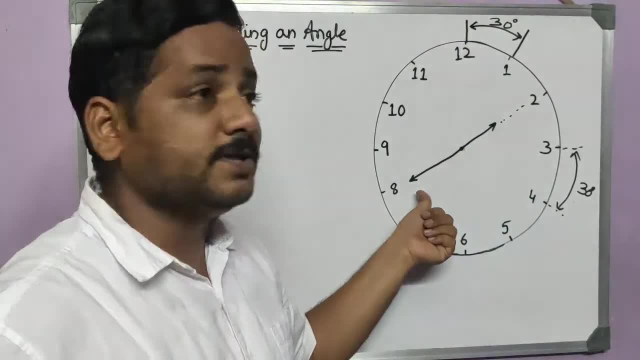 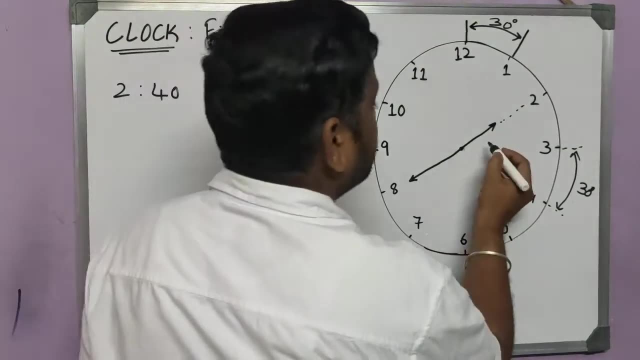 Because it is 2 o'clock for 2 hour and 40 minutes, So this is not exactly at 2.. Now this hour hand will be almost Closer to the 3 o'clock Okay, So somewhere here. 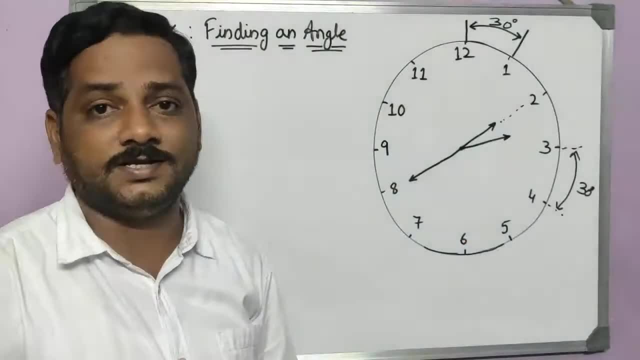 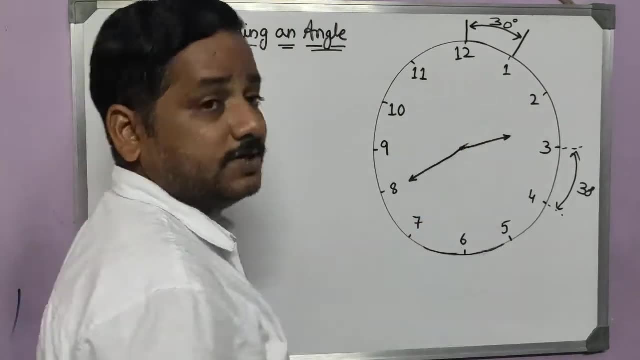 You get somewhere here. So it is in between 2 and 3.. But we do not know what is the exact angle. Okay, So that is what you need to calculate, You need to find now. So this is first thing you need to understand. 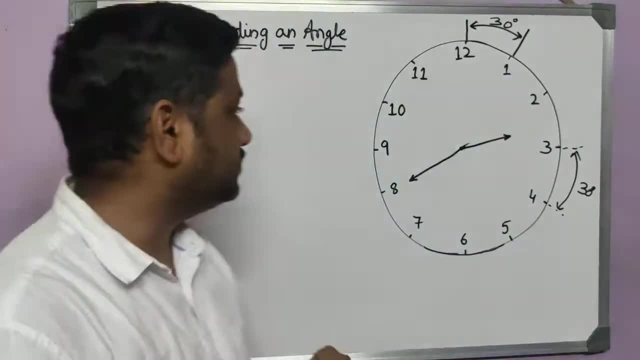 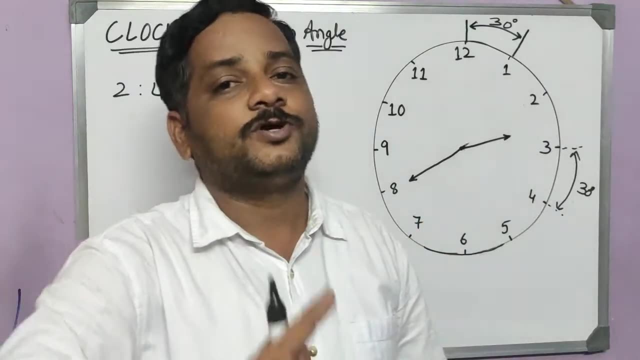 Whenever you plot this, Whenever just you need to make an imagination: 2 hour and 40 minutes. in the sense It is more than 0 minutes, So hour hand will not be pointing towards that exact time- 2 o'clock, Isn't it? 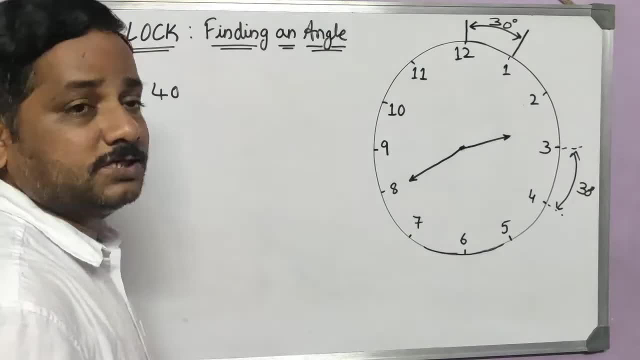 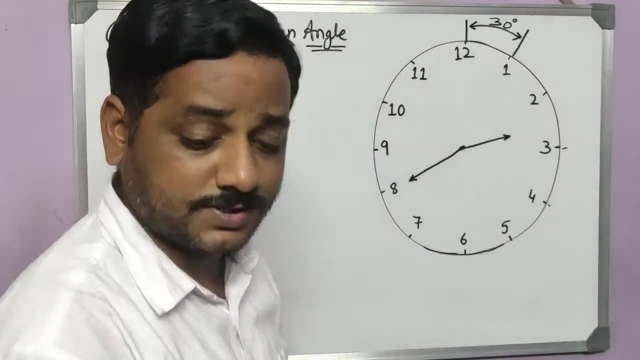 Now this is what we have: 2 hour and 40 minutes. The question is to find the angle between these two hands. Now how to find it? Use first note. What is first note says? Note 1 says that The each sector is going to have 30 degree. 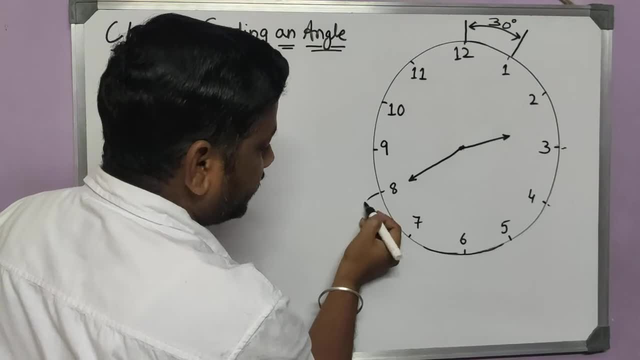 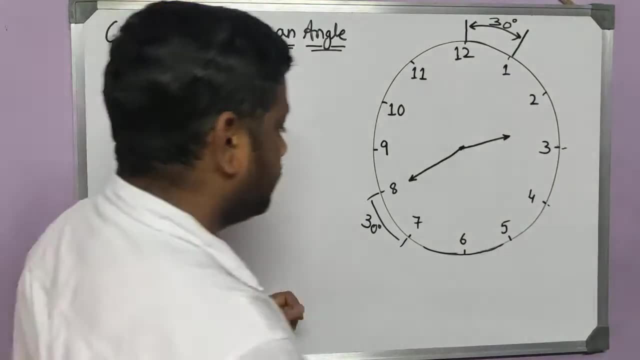 And here, what are the sectors we are getting in between these two? See from 8. We have from 8 to 7.. So this is one sector wherein I can consider this as 30 degree, And this is the another sector coming in that. 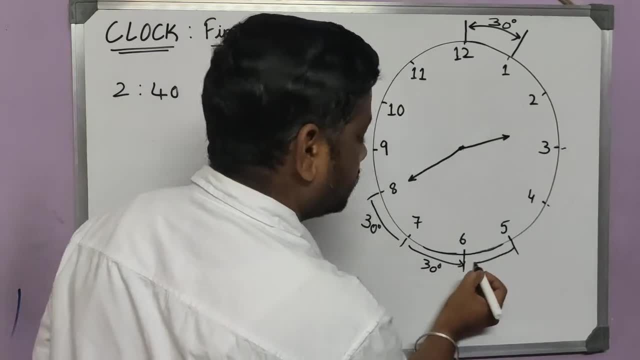 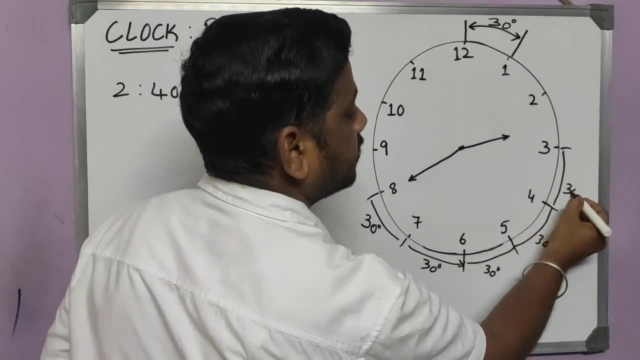 So 30 degree Plus 30 degree Plus. we have another sector here: 30 degree. So we have the another sector. This is also 30 degree. Even this is also 30 degree. Right, But now you cannot consider this sector from 2 to 3.. 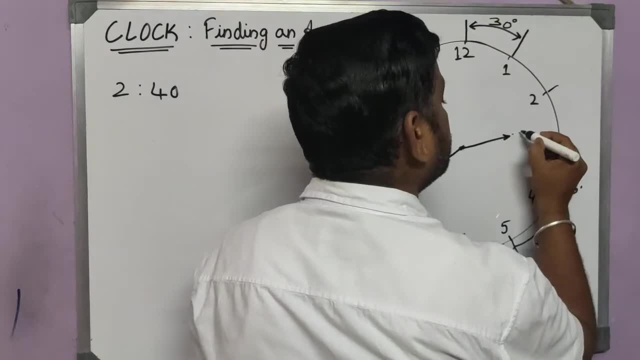 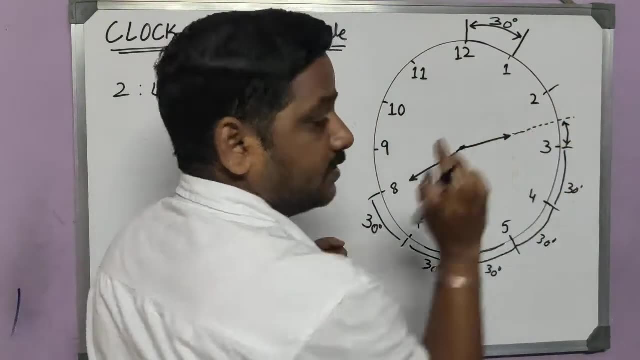 Because hour hand is not exactly at 2. It is in between the 2 and 3. So this degree you need to identify. So we do not know this. We know complete angle between 2 and 3 is 30 degree. 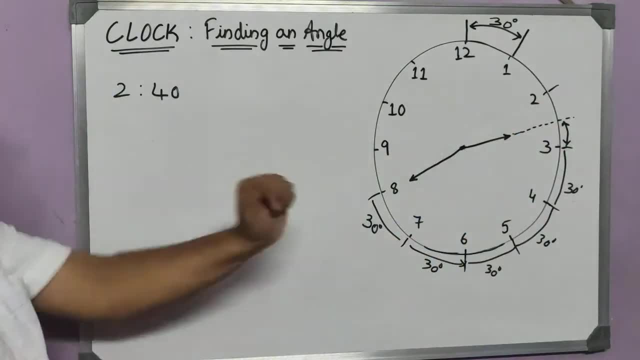 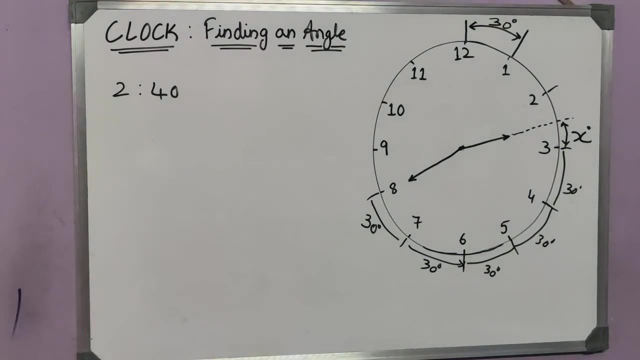 But now I want to find. I want to find only this portion, and remaining portion is already obtained. So let me consider this as x degree. We do not know that, So that is an unknown angle To find this. let us see what is the next concept. 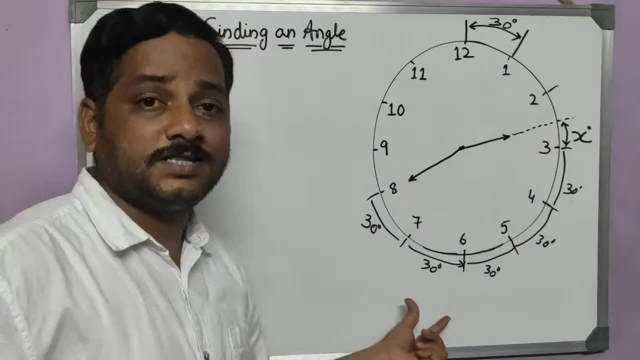 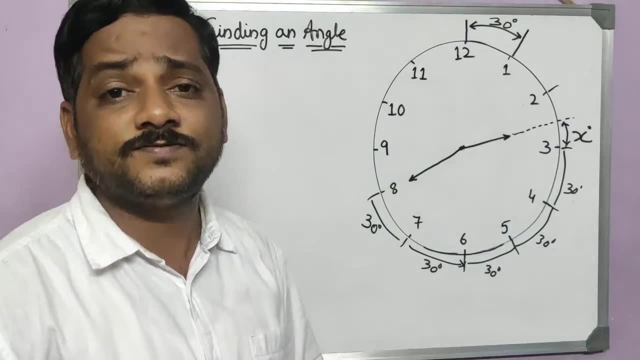 So here I just make use of a first point, That is, each sector is having an angle of 30 degree. 1, 2,, 3, 4, 5. So 5 into 30. So we get 150 degree. 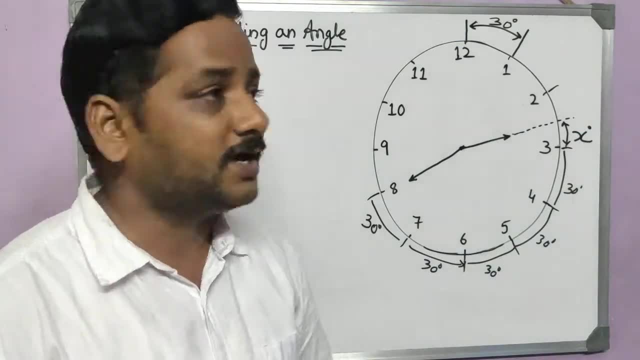 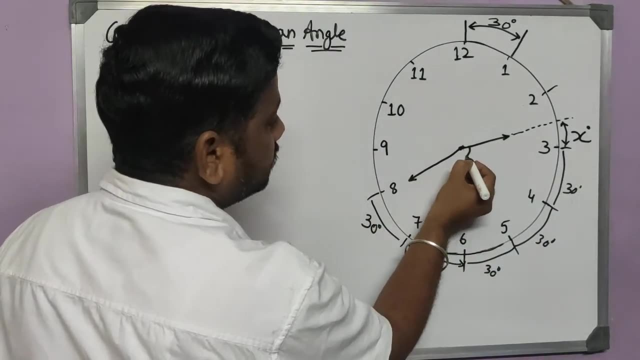 150 degree plus this x degree will give you an answer for an angle between the 2. Hand to hours To hand, ands. So this is an angle, So this is theta. So how to find this x degree now 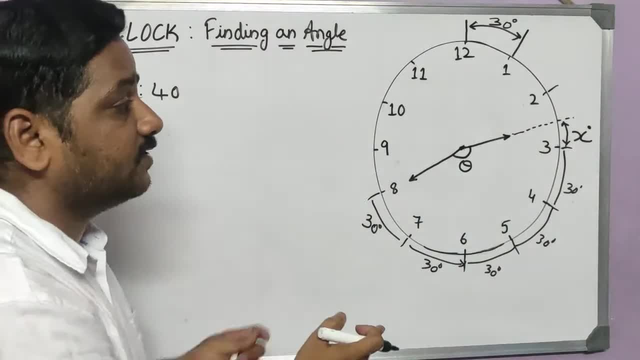 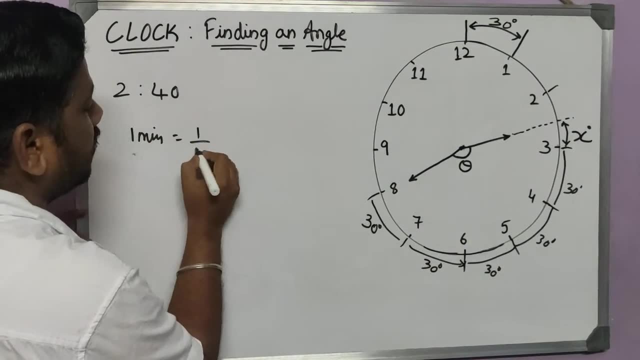 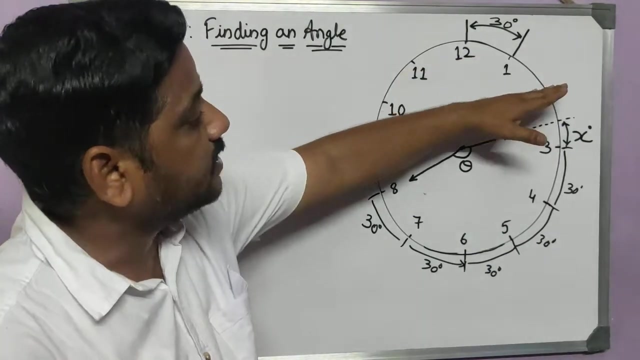 See one thing you can identify here. Now I will make use of a note 2.. So note 2 says that 1 minute will be equal to half the degree. Right, So here this and hour is away from 2 and near to 3.. 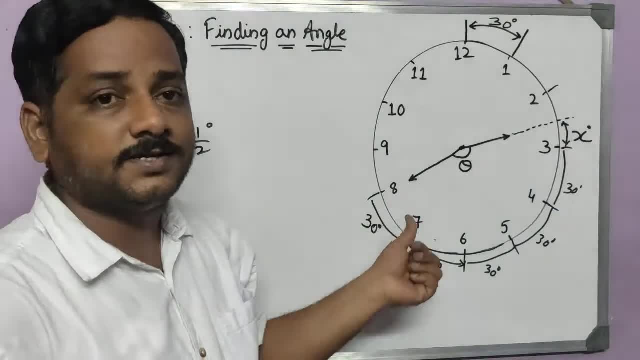 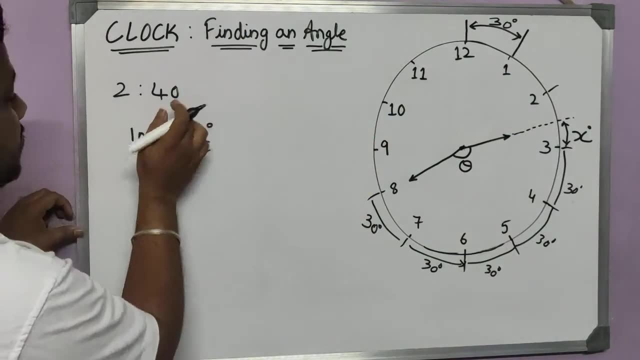 And how many minutes has been happened. now It is 40 minutes, So for 1 minute we have half a degree of an movement of an hour and hour, Okay Hour, and So now it is 40 minutes. So for 40 minutes, what you can say? 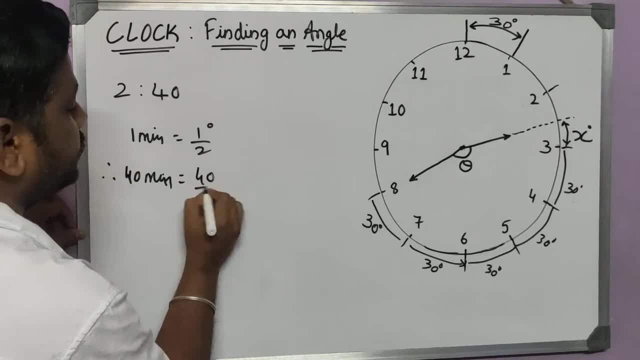 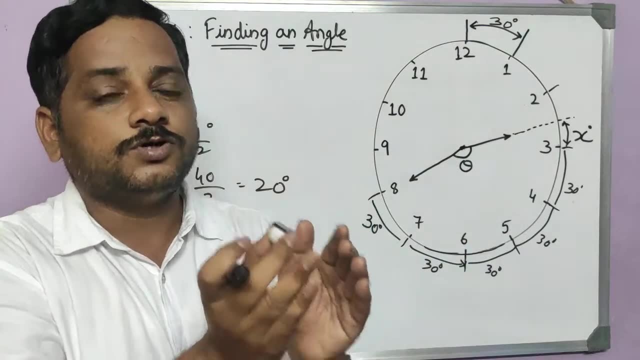 For 40 minutes. therefore, for 40 minutes it will be 40 by 2. That is nothing but 20 degree. So I can say that our hand has been moved 20 degree towards 3 o'clock. It is moving towards 3, right. 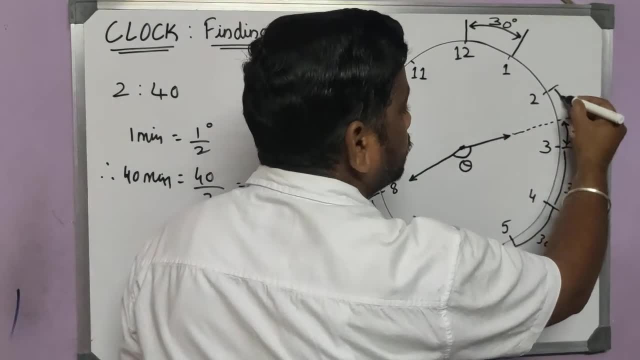 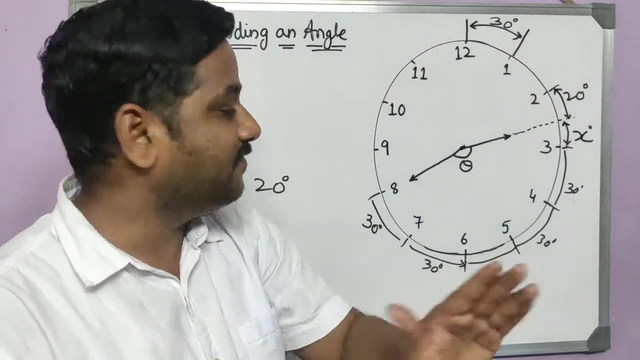 So 20 degree means it is moved from 2 to 3 o'clock at 20 degree. So this portion is 20 degree, not the x We are trying to find what is the position of an hour hand. So it has to be at 2 to 3.. 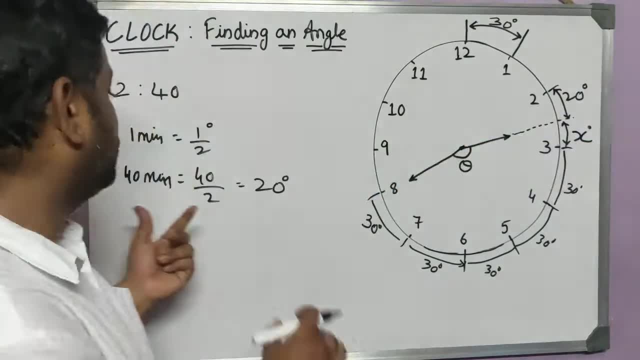 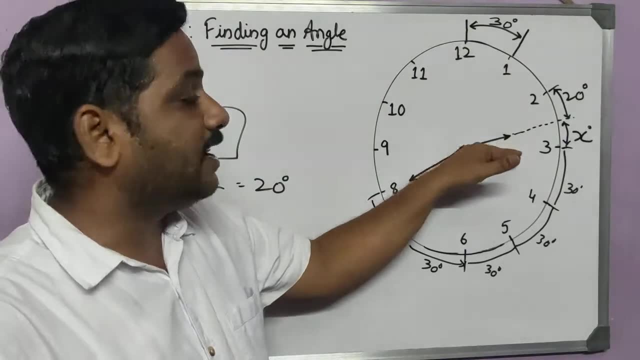 It is moving from 2 to 3.. So we are finding this portion now Using this note 2, using this formula, we can find what is an angle. the hour hand has been moved, So it is moved by 20 degree. 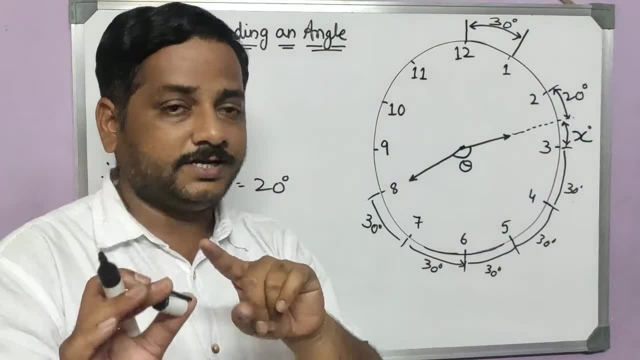 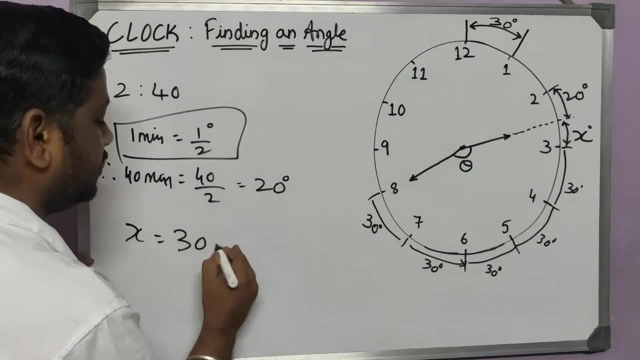 So we can say the total angle of this sector was 30 degree. Now already it has moved 20 degree. So x will be just it will be. x can be taken as the total sector angle minus that angle, 20 degree. 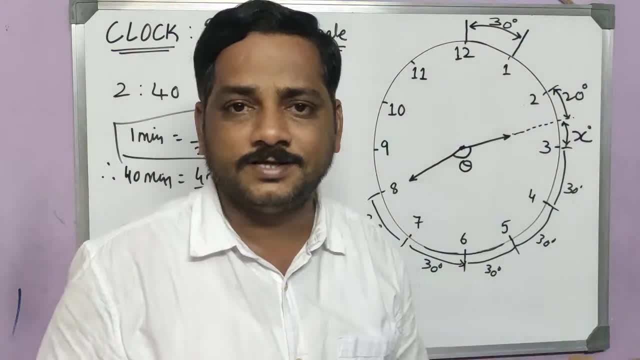 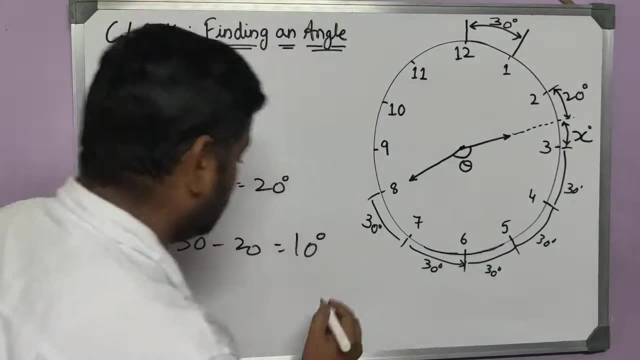 It is 10 degree, So x is equal to 10 degree, right, So now we can say 30, 30,, 30,, 30, 30. So 5 times, So 150 plus 10.. 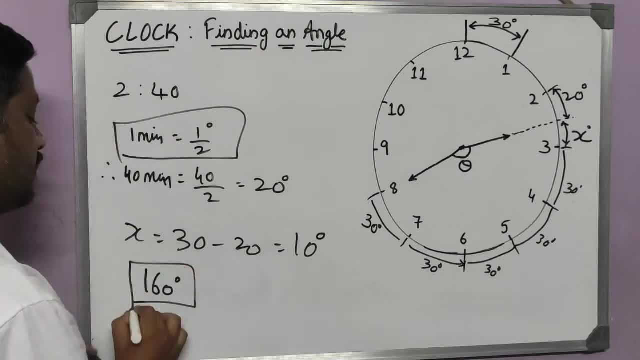 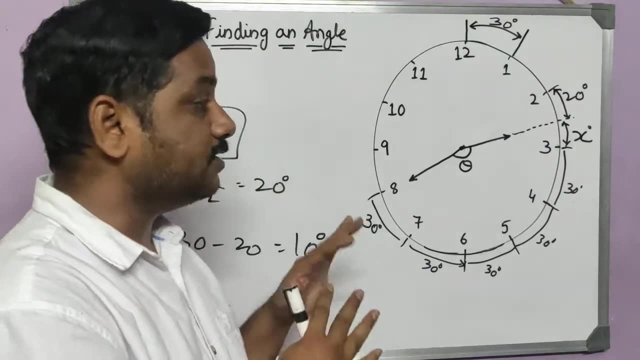 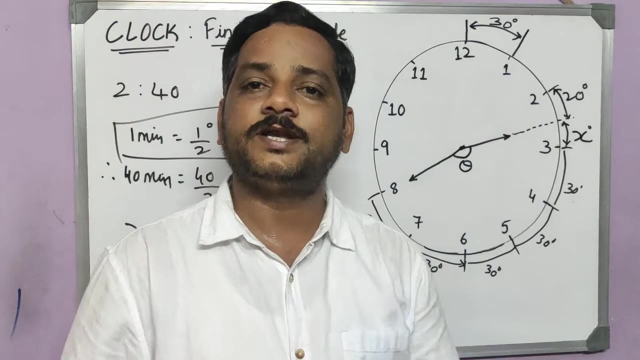 Therefore, the angle between the hour hand and the minute hand is 160 degree. I hope it is clear, See. if the concepts are clear for you, then press the like icon here, And if you want to feel to share something about this video, put it in a comment box. 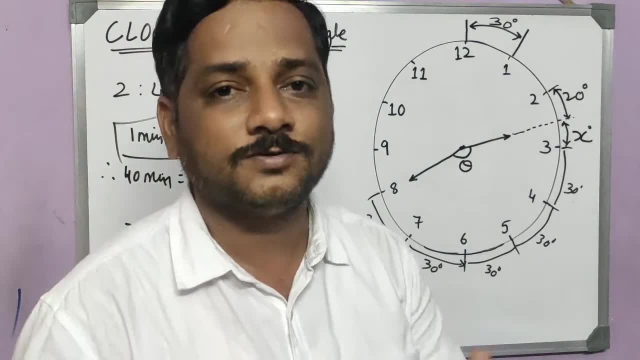 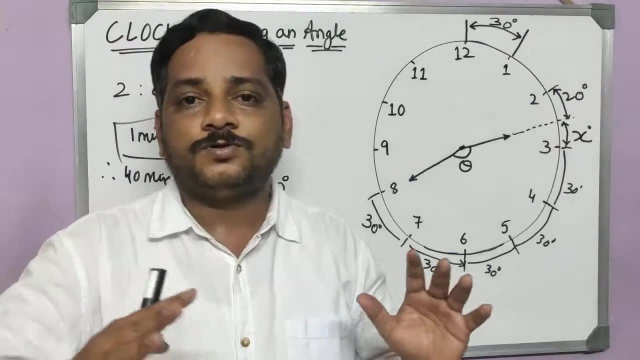 And also you want to get any other videos, you just put it in a comment box so that I can also make a video on those topics. I think this is very clear for you guys. So here I don't want to give one more example here, because this is just a basic video on the clock. 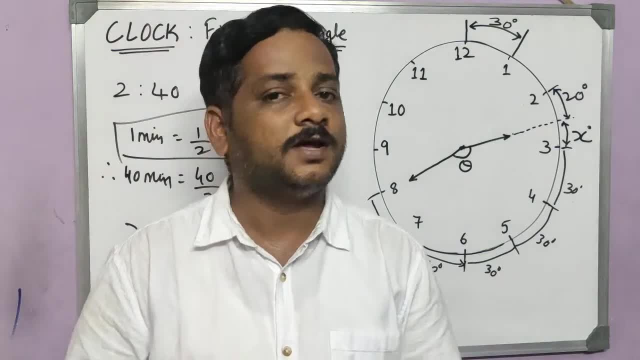 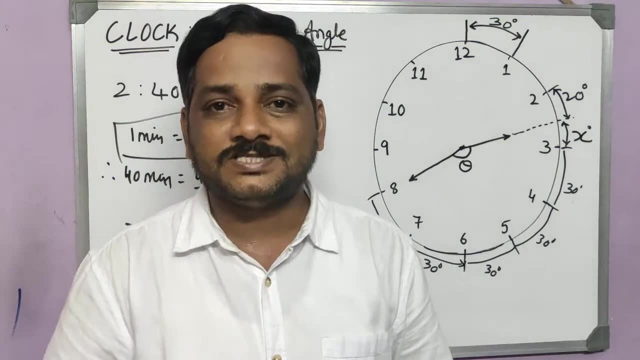 So in next videos I am going to come up with some more questions and some more new topics. If it is clear for you and you have an interest to learn, then please subscribe to my channel so that you can get a notification whenever I upload a new video. Thank you.